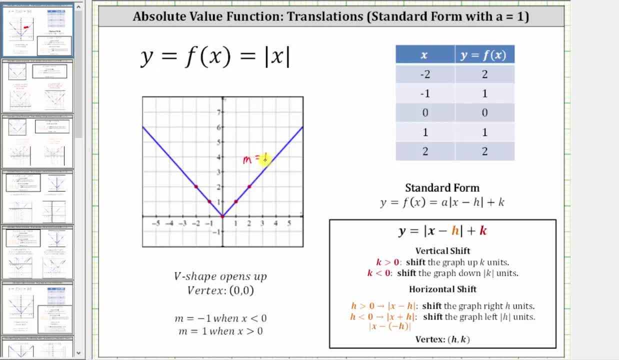 on the right side and go up one and right one, we can determine another point on the graph And then, when x is less than zero or to the left of the vertex, the slope is negative one. Now, going back to the form of the equation, y equals: 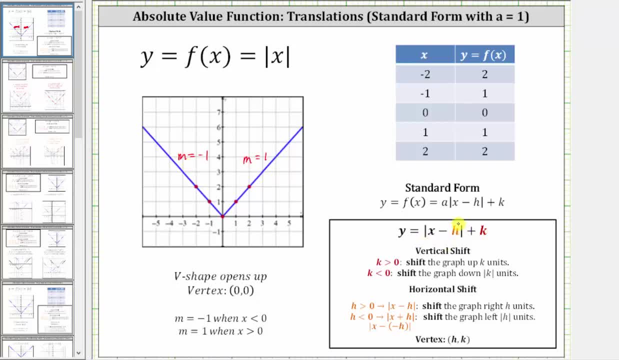 the absolute value of the quantity x minus h plus k. the value of the quantity x minus h plus k. the value of h will shift the graph left or right and the value of k will shift the graph up or down When h is positive or greater than zero. 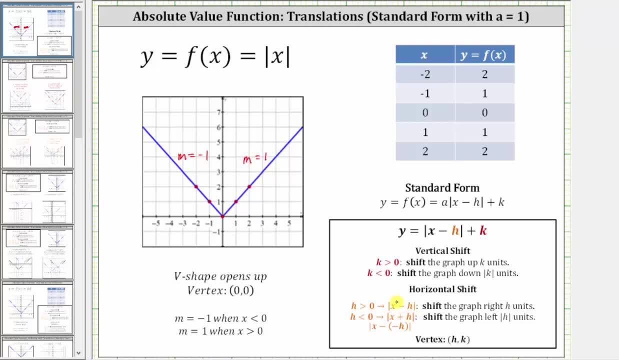 we would have the absolute value of x minus h. so when we have subtraction here, h is positive and the graph is shifted right, h units And when h is less than zero or negative, we would have the absolute value of the quantity x minus negative h. 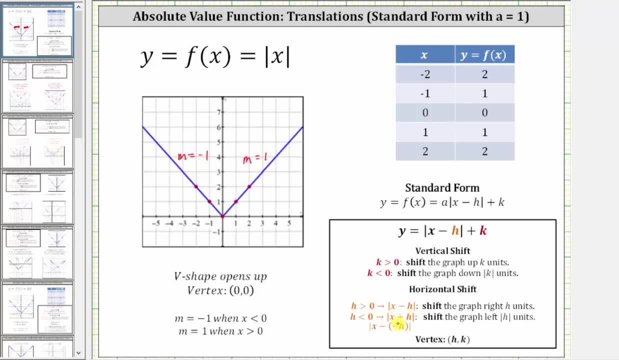 which simplifies to x plus h. so when we have addition here, h is negative and the graph is shifted left: the absolute value of h units. And now for k, when k is positive or greater than zero, the graph is shifted up: k units. 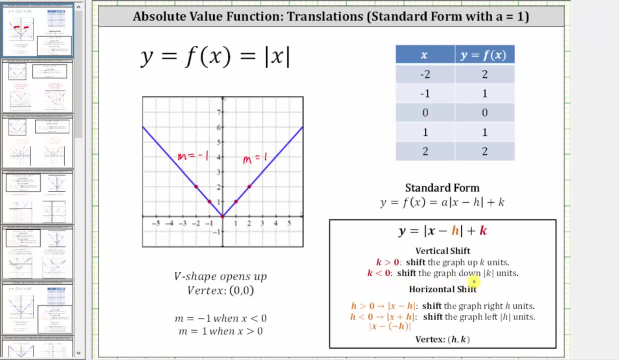 and when k is less than zero or negative, the graph is shifted down. the absolute value of k units And then, finally, the vertex is the ordered pair: h comma k. Let's look at an animation to better understand how the values of h and k affect the graph of the basic. 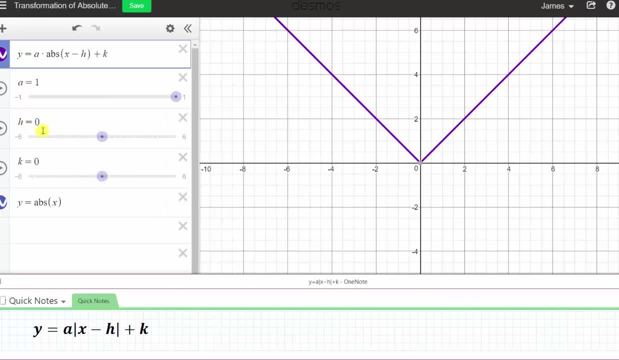 Let's first see how h affects the graph of the function. Notice: when h is positive, the graph is shifted right- h units- and when h is negative, the graph is shifted left- the absolute value of h units. So if we stop here for a moment, 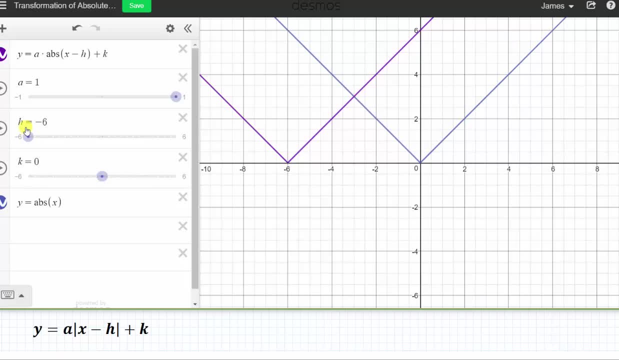 where h is negative six. let's determine the equation of this graph. Well, if h is negative six and we know a is one and k is zero, this would give us the equation: y equals the absolute value of the quantity x minus negative six. 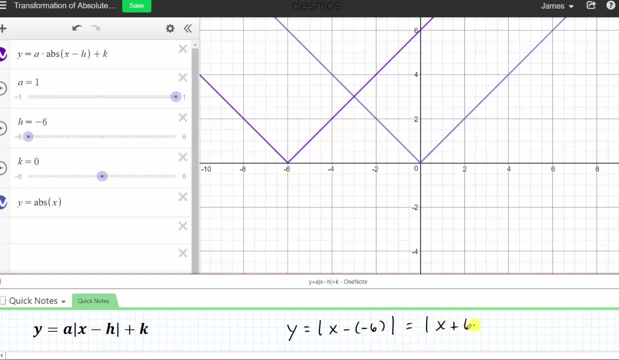 Simplifying, we have the absolute value of the quantity x plus six. So again, when we have addition inside the absolute value, the graph is shifted left, in this case six units. And this should make sense, because notice how, when x is negative six. 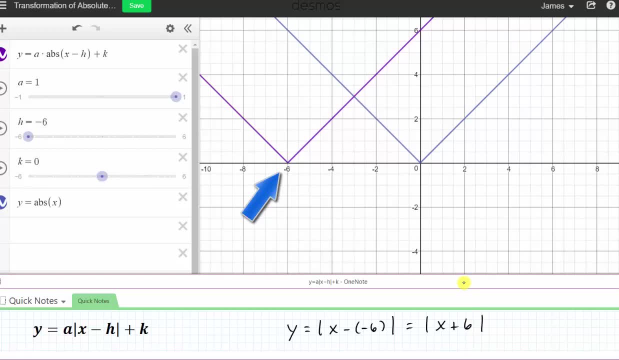 the ordered pair. here the vertex is negative six, comma zero. and, notice, when x is negative six, we do have a zero inside the absolute value. the absolute value of zero is zero and therefore the output, or y value, is zero when x is negative six. 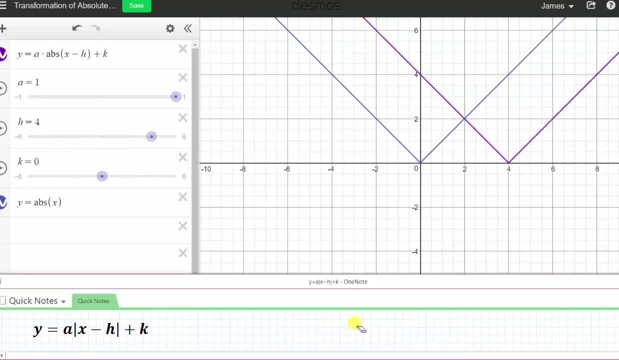 And when h is positive, let's say when h is positive four, we would substitute positive four in for h, which gives us the equation: y equals the absolute value of the quantity x minus four. Again, when we have subtraction inside the absolute value. 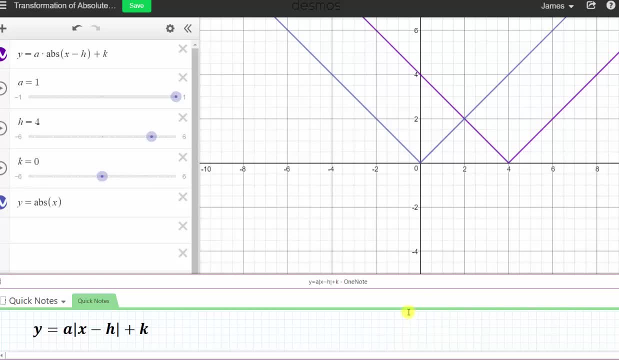 the graph is shifted right, in this case four units. And now let's see how k affects the graph. So we'll say that h back to zero, and now change the value of k. Notice, when k is positive, the graph is shifted up k units. 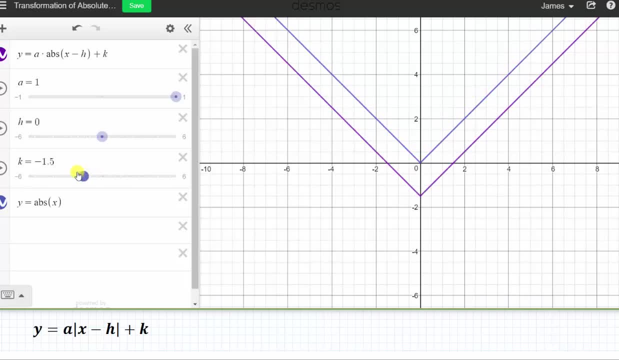 and when k is negative the graph is shifted down. the absolute value of k units. So here, where k is equal to negative four- because we have addition here, we normally don't write plus negative four, we normally just write minus four. 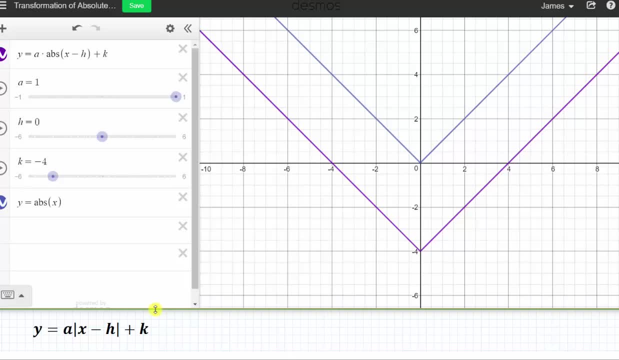 And we know a is one and h is zero and therefore the equation of this purple graph is: y equals the absolute value of x, and then minus four. And let's take a look at an equation: when k is positive, Let's change k to positive two. 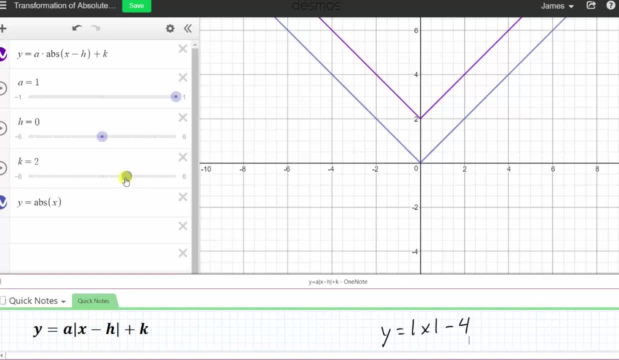 Notice how the graph is shifted up: two units and because k is positive two, the equation of this purple graph, or this graph here, is: y equals the absolute value of x plus two. Let's take a look at a few more examples. Let's say we're asked to graph y equals. 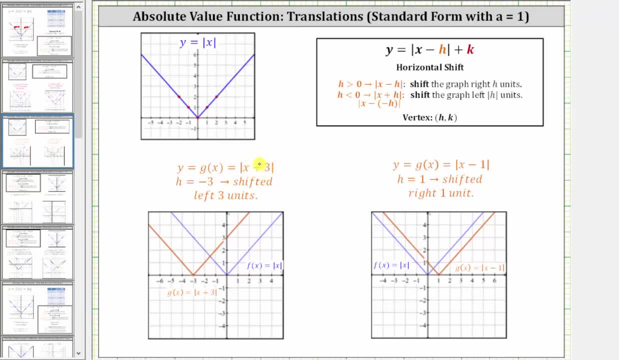 or g of x equals the absolute value of x plus three. Again, because we have addition here, h is going to be negative three. we need to be thinking that we can write x plus three as x minus negative three to determine the value of h. 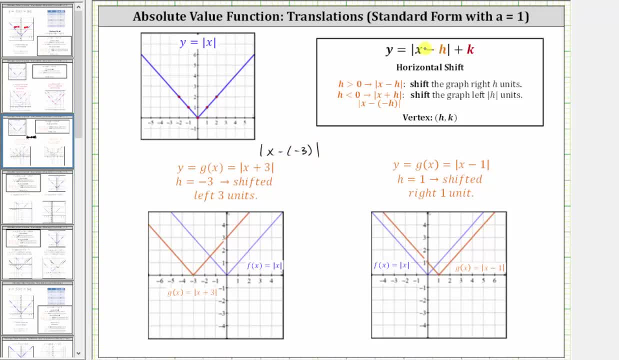 Again because in standard form we do have subtraction inside the absolute value. So because h is negative three, the graph is shifted left the absolute value of negative three or three units, And so notice how the graph would be, this orange graph here.